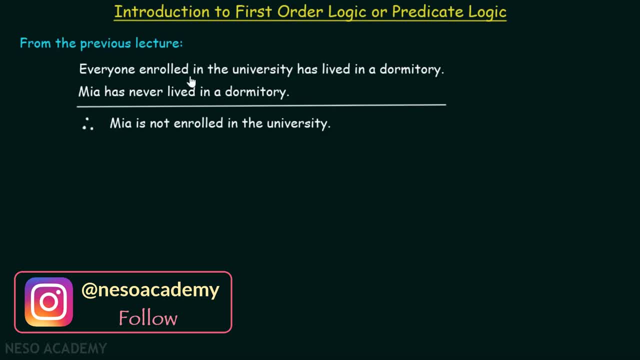 In the previous lecture, we have seen this argument that is everyone enrolled in the university has lived in a dormitory. Mia has never lived in a dormitory. Therefore, Mia is not enrolled in the university. We have seen that propositional logic is not capable enough to handle these type of arguments, right? That is why we have moved to first order logic. 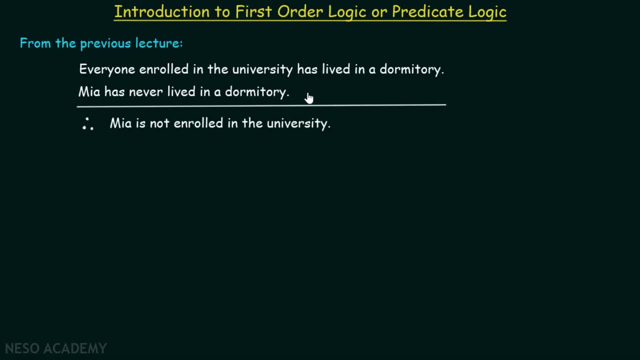 First order logic has the capability to handle these type of arguments. Basically, these type of arguments could not be handled by the rules of propositional logic. 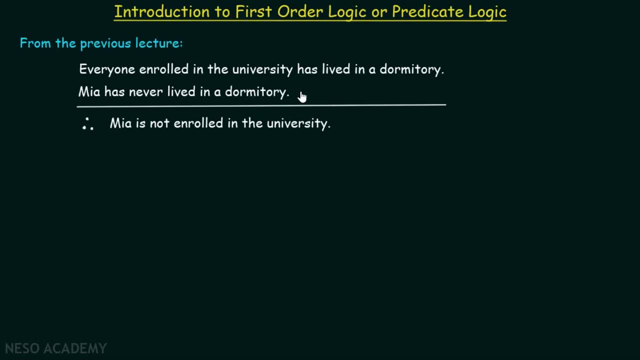 That is why we will go one step further. That is, we will identify the validity of these type of arguments using first order logic. 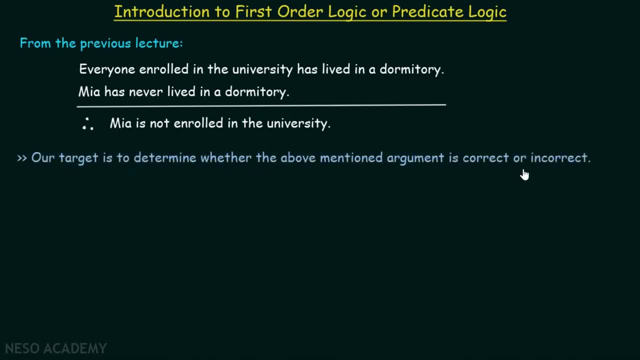 Our target is to determine whether the above mentioned argument is correct or incorrect. This is the primary target. For this, we should understand predicate logic or first order logic. And in order to understand predicate logic, we must understand the following. 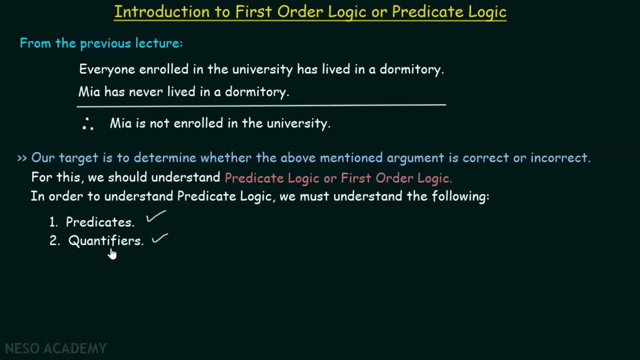 That is, predicates and quantifiers. And that is why we are dealing with them. 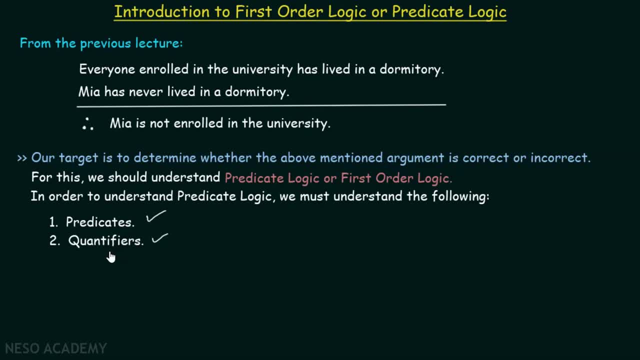 First, we will understand what are predicates and then we will understand what are quantifiers. 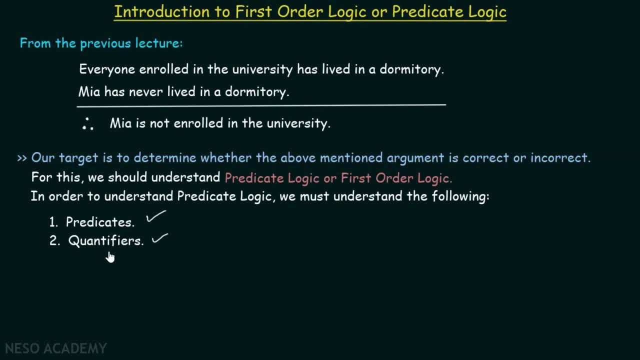 In this particular presentation, we will understand what are predicates and in the subsequent presentations, we will understand what are quantifiers. Here comes the definition of predicates. 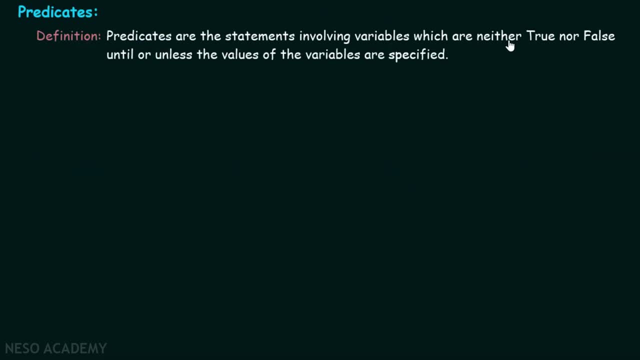 Predicates are the statements involving variables which are neither true nor false until or unless the values of the variables are specified. 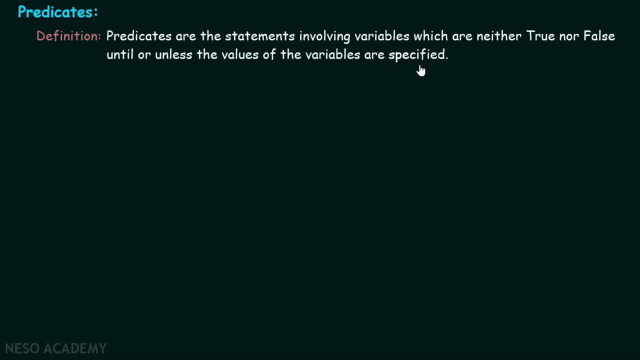 So, this is the definition of predicates. Predicates are basically the statements involving variables which are neither true nor false until or unless the values of the variables are specified. We will consider certain examples here. 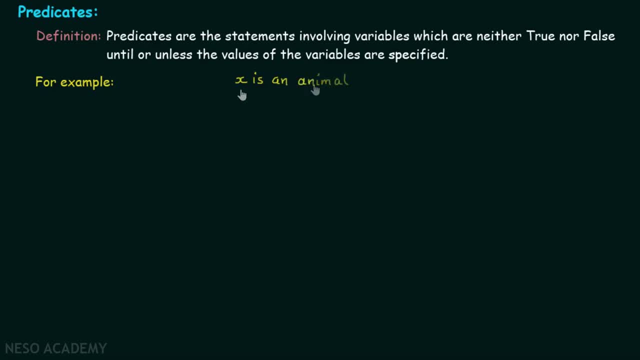 Let's say that x is an animal. This statement involves a variable. That is why we cannot identify the truth of this statement until or unless we will give the value to this variable. 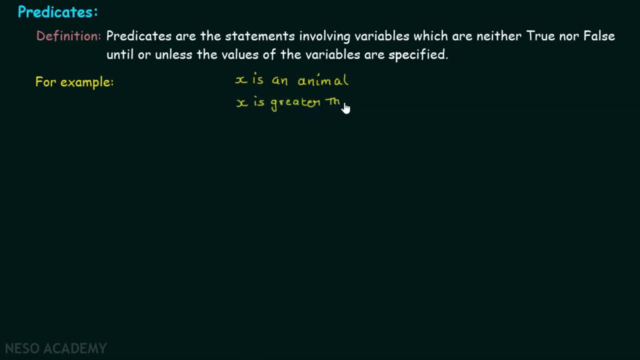 Or we could have something like this. x is greater than three. We could have something like this also. 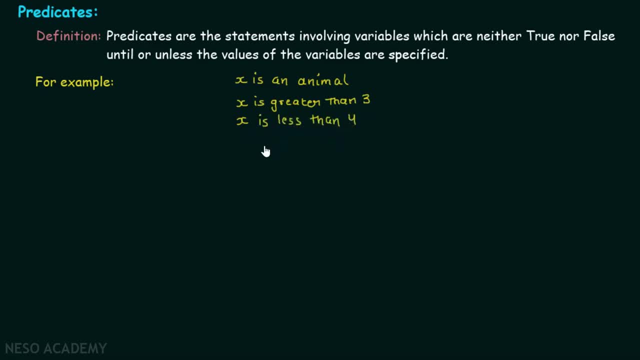 x is less than four. Or we could have something like this. x plus y is equal to seven. 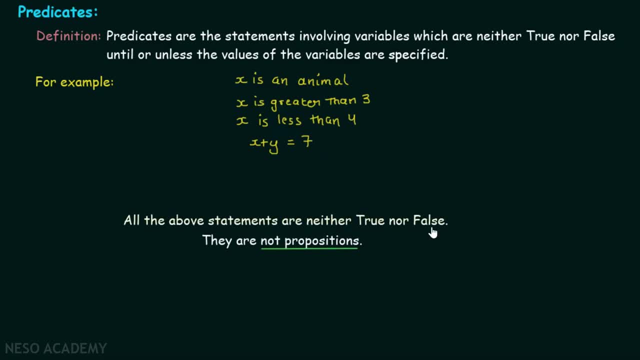 All the above statements are neither true nor false. They are not propositions. Because we cannot identify the truth value of these statements, that is why they are not propositions. They are simply the statements. 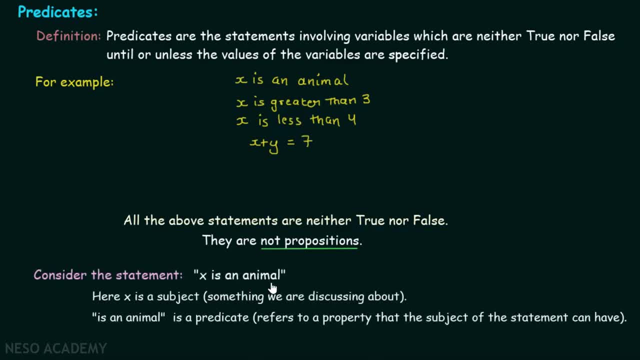 Now, I want you to consider the following statement. That is x is an animal. Here, x is a subject, right? Something we are discussing about. 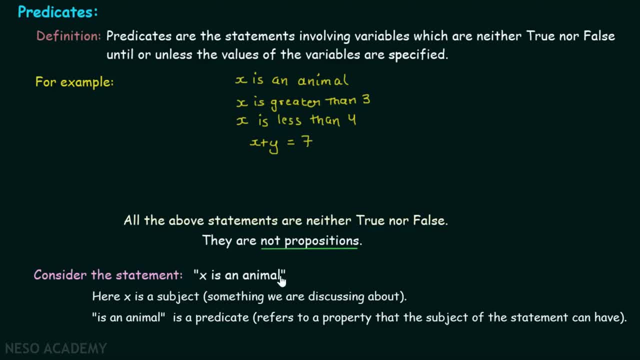 Here, this is a subject and this is a predicate. Is an animal is a predicate. Because it refers to a property that the subject of the statement can have. 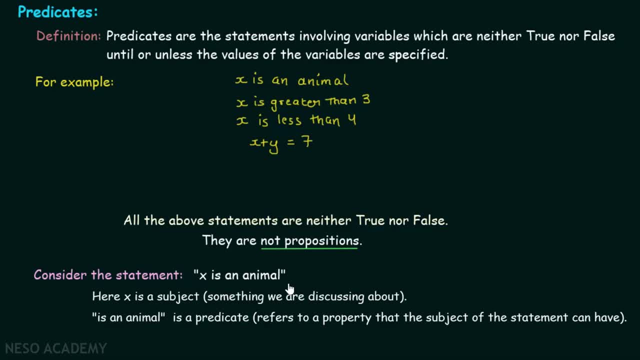 So, x is basically representing a subject and this represents a predicate. In predicate logic, a statement is divided into two parts. 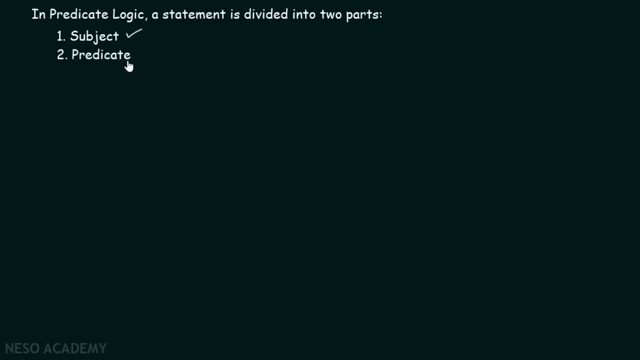 The first part is subject and the other part is predicate. Usually, we denote such statements with a shorthand notation. 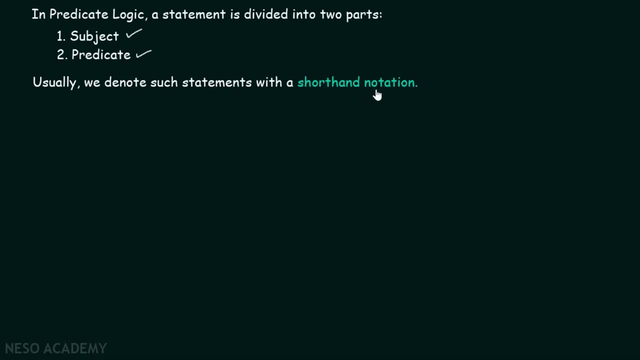 It should be well noted that we denote such statements with a shorthand notation. 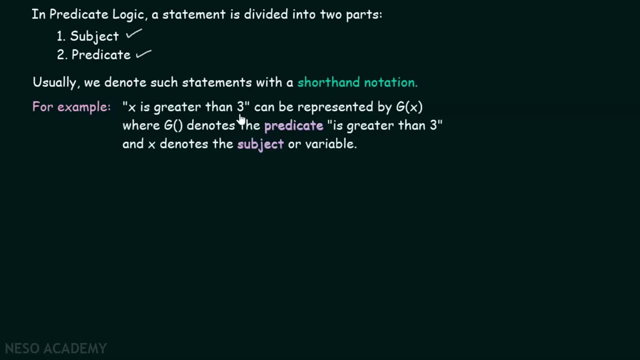 For example, here we are considering this statement x is greater than three. This can be represented by gx where g denotes the predicate is greater than three and x denotes the subject or variable. Okay, here this is the subject and is greater than three is a predicate. So, it is clear from this fact that first part of the sentence is a subject which we are talking about and the second part is the predicate that represents the property of that subject. 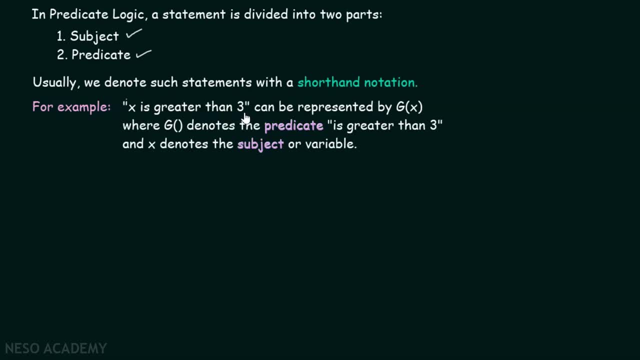 So, this is the basic idea of predicate logic. Here the statement is divided into two parts. 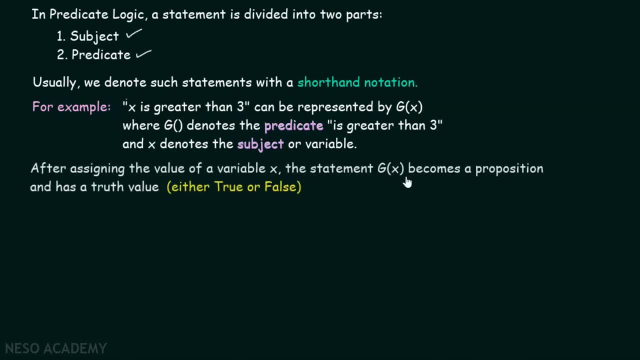 After assigning the value of a variable x, the statement gx becomes a preposition and has a truth value. Either it could be true or false. Right now, we cannot identify the truth value of the statement because we don't know what is x. But after assigning the value of x, we can identify the truth value of the statement. 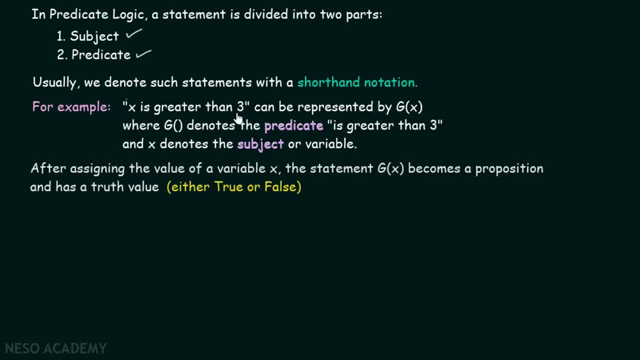 This is very important. Here you can see this statement is represented using this gx, this shorthand notation where g represents the predicate and x represents the subject, right? 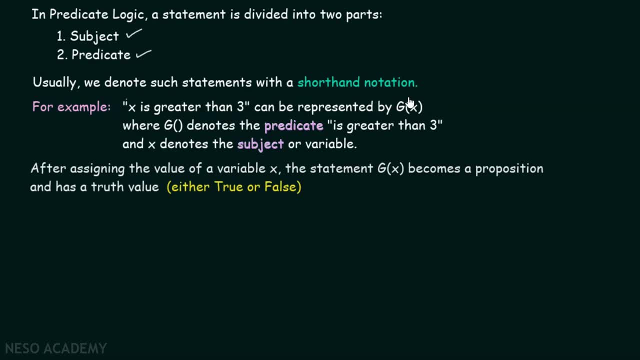 So, here this shorthand notation is very useful. We can use these shorthand notations later in order to perform operations because we can't write these statements again and again. 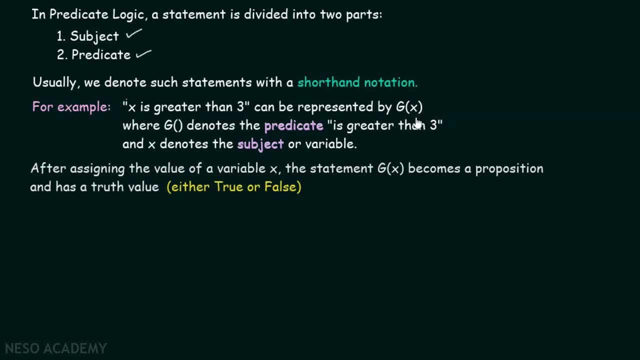 That is why we represent them using these shorthand notations. Let's see certain examples of how to assign a value to a variable x. 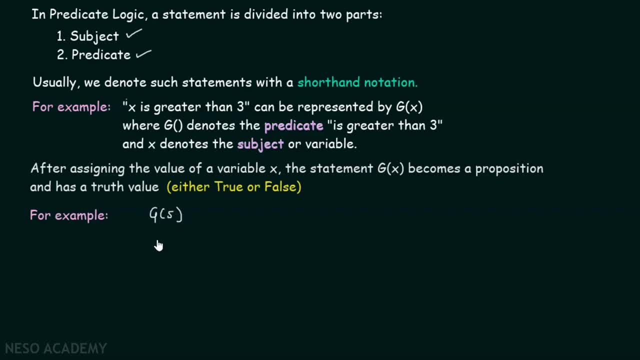 Here let me consider something like this, g5. What do you think? What is the truth value of g5? 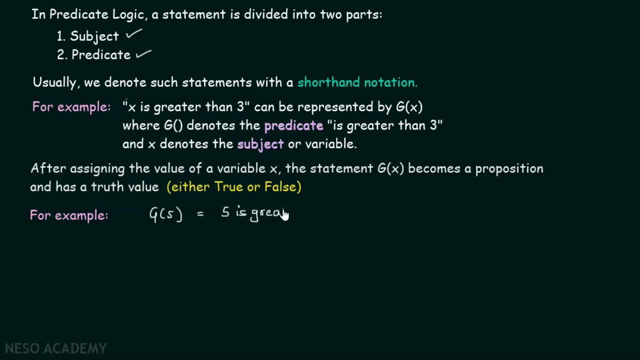 g5 basically represents that 5 is greater than 3. Isn't that so? 5 is greater than 3 is the representation because here x is replaced by 5. 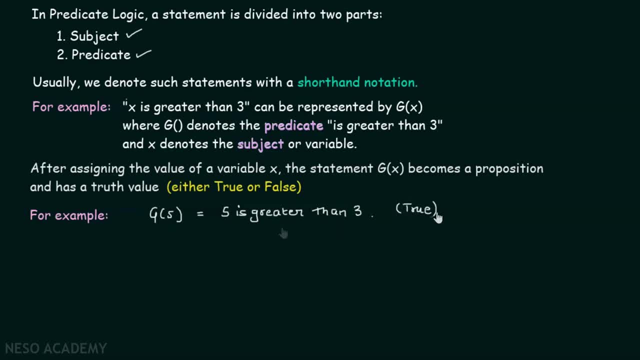 5 is greater than 3 is true. Isn't that so? 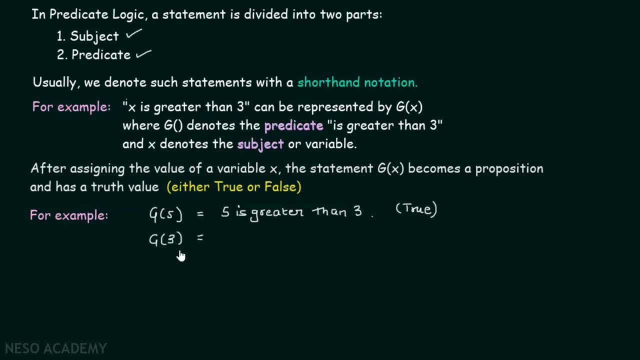 Now, if I give you something like this, g3. What do you think? What is the truth value of the statement? 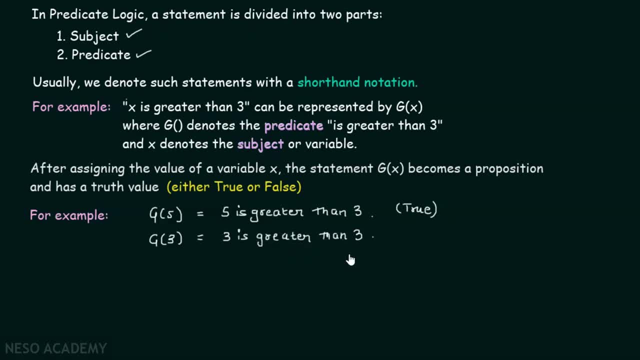 3 is greater than 3. Is it true? 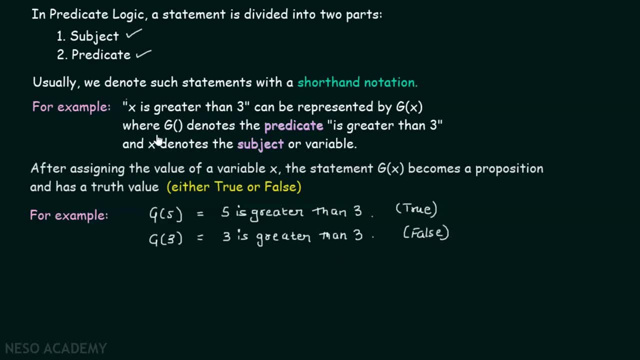 No, it is not true. We can see that after assigning the value of x, we will get the truth value of the statement, right? Either it could be true or false. Now, it depends upon the value of x. Okay friends, this is it for now. 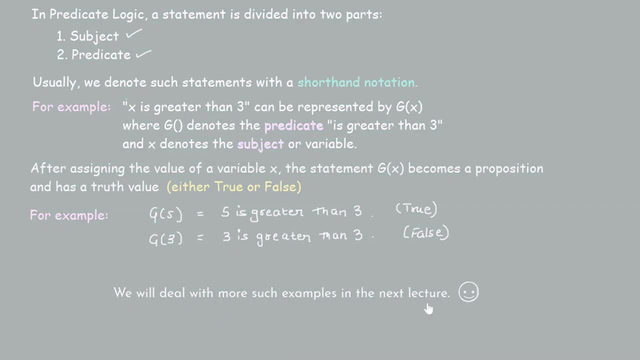 We will deal with more such examples in the next lecture. 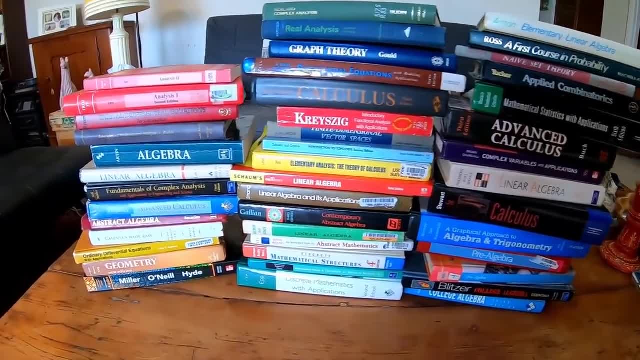 Hi everyone, in this video I'm going to show you how to teach yourself mathematics from start to finish, starting with just like basic sets and proofs. So we'll start with actually learning to write proofs and learning some logic and a little bit of discrete mathematics, and then from there. 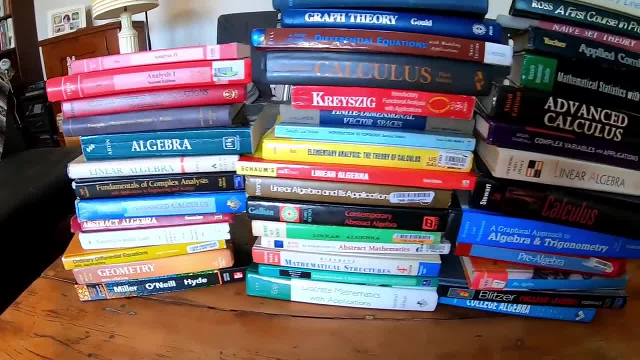 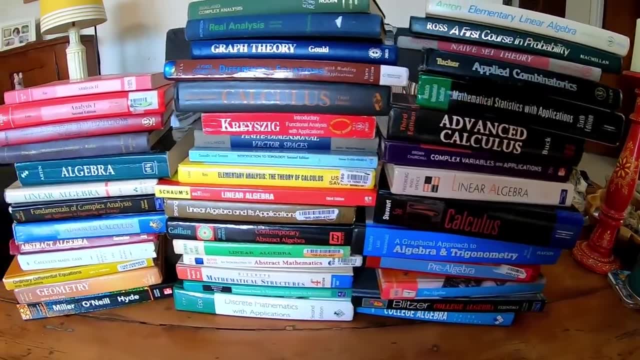 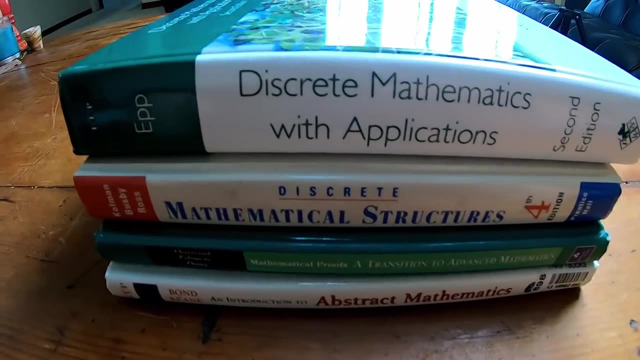 in theory, you could teach yourself tons of mathematics. I'm going to show you the exact order that you should follow, or at least a highly recommended order. Let's get started right away. Okay, so here I have four books that I think are a really, really good starting point. So the first: